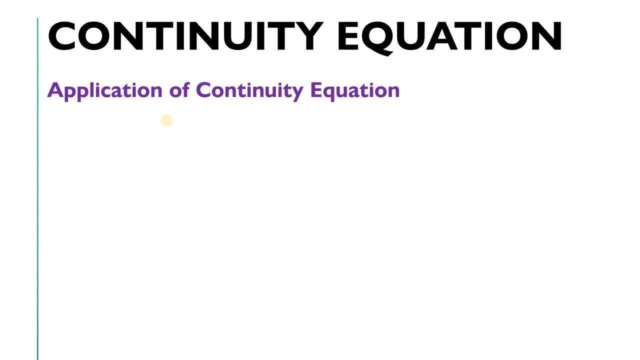 and after that we will discuss about the application of this continuity equation. If we are reading the continuity equation, we are studying the continuity equation here, So what is the application of it If you are an engineering student, if you are an engineer in any plant, or if you are right now? 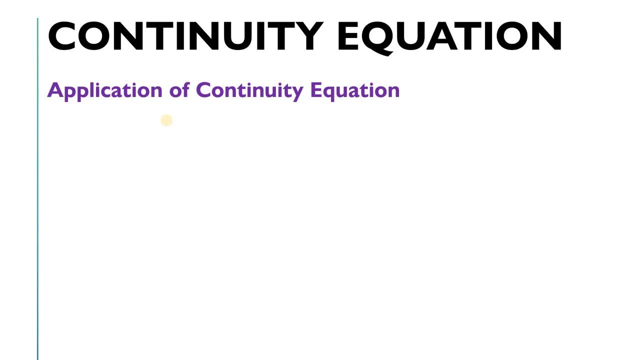 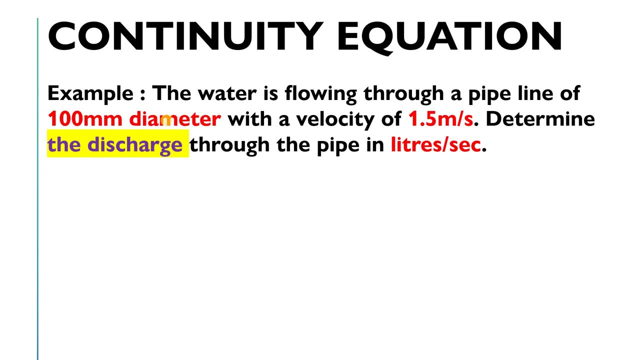 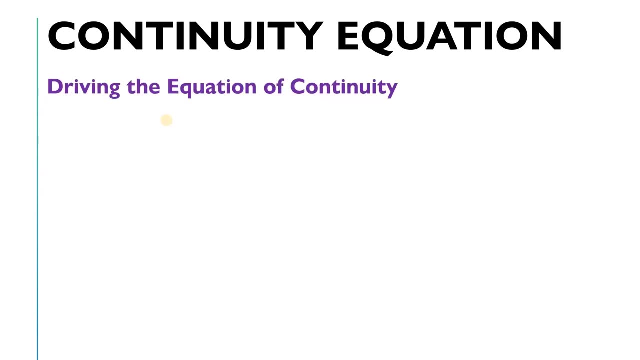 the student in your like, let's suppose, in your secondary higher education. So you must know about it. And in the last we will discuss about the this example. So we will calculate the discharge flow rate here with the help of the our given data. Got it my point, So now let's start the. 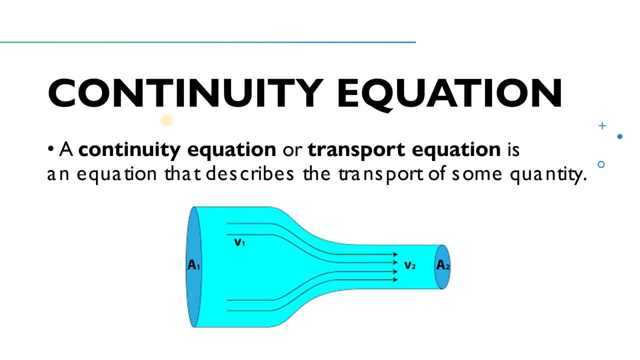 continuity equation. with what is continuity equation, Continuity equation or a transport equation? It is also known as the transport equation. Okay, So, as the name consists transport, it means that it is transporting something. Transporting means from one side or one location to another location, Let's suppose from one to from two, Right And. 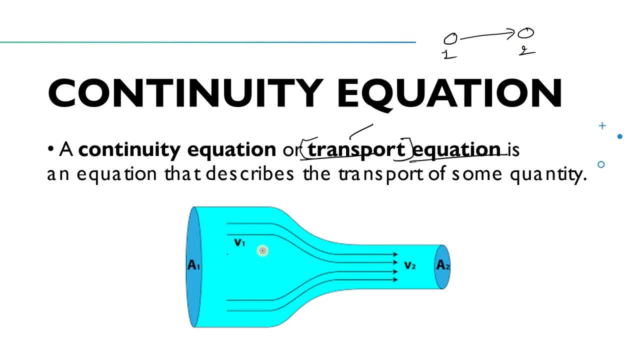 here also you can see that your fluid is flowing. Let's suppose your fluid is following from A1 cross sectional area. Okay, This is your area A1. Right From A1 cross sectional area to A2 cross sectional area. So continuity equation is an equation that describes the 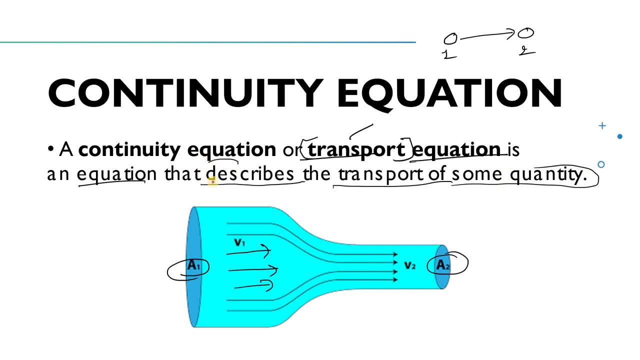 transport of some quantity. So what it is telling you, it is describing or it is giving us the useful information about the transportation or transport of some quantity. Or simply you can say: transport of fluid. Right, It may be your gas or it may be your liquid. Got it, my points? This? 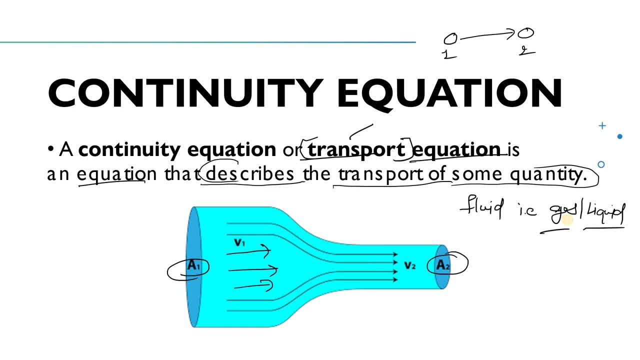 is the generic information about the continuity equation. Actually, what is the continuity equation? Okay, This is the. actually, this is the transport equation, Okay, Which describes about the transport of some quantity. Now, if we discuss about the definition of the continuity equation, or simply, 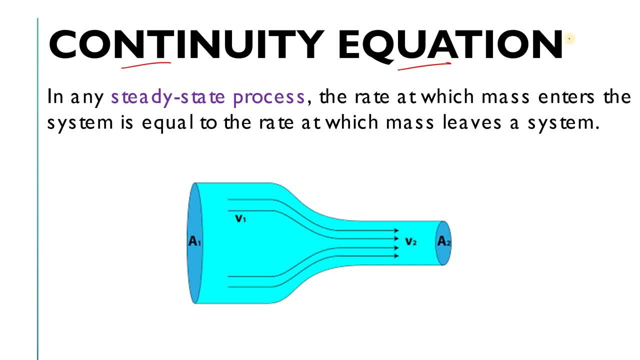 say the statement of the continuity equation, what the quantity equation says in fluid dynamics. Here, whatever we are discussing, that we are discussing with respect to fluid dynamics or fluid mechanics, you can say: Right, Okay, so let's discuss about the statement of the continuity equations. So it 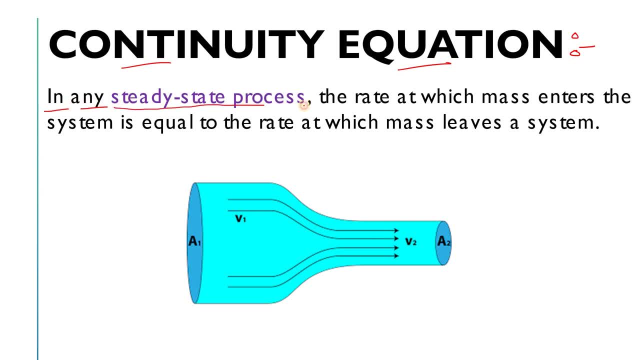 states that in any steady state process, okay, it means your process is steady state, Right, taking the assumption that it is a steady state process. but you will see that in industries or in your daily life, example, the steady state process are mainly not possible. right, because we, we always 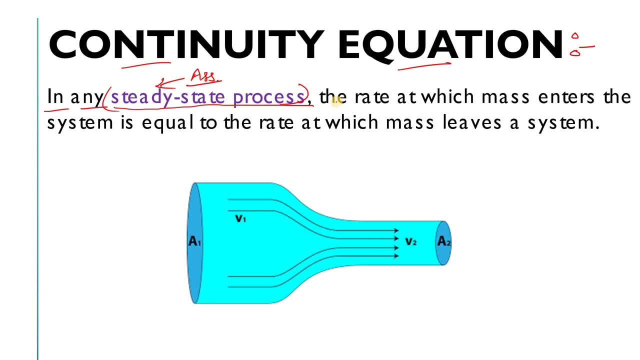 deal with the unsteady state process in our practical life. right? so the weight at which mass enters the system- okay, is equal to the weight at which mass leaves the system, or leaves a system- okay. what is it means? it means that your mass is going to be conserved here. so whenever we 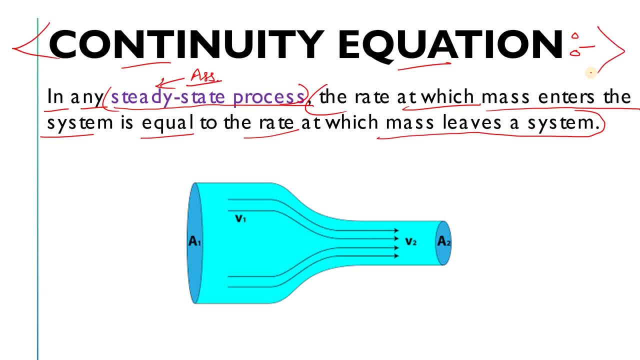 discuss about the continuity equation. so the conservation quantity comes into the picture. let's suppose here we are discussing about the continuity equation with respect to fluid mechanics. so the mass will be conserved here. okay, let's suppose your fluid is flowing from here to here. right, your fluid is flowing like that, the direction is like that, right? 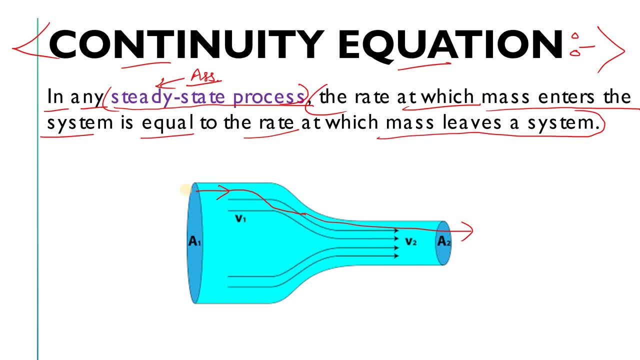 so what it is saying? that the mass will be conserved means mass cannot be create. mass can neither be create nor destroyed, same as energy, right? so your total mass will be, your total mass will be conserved here, right? so this is the your continuity equation. okay, so this? 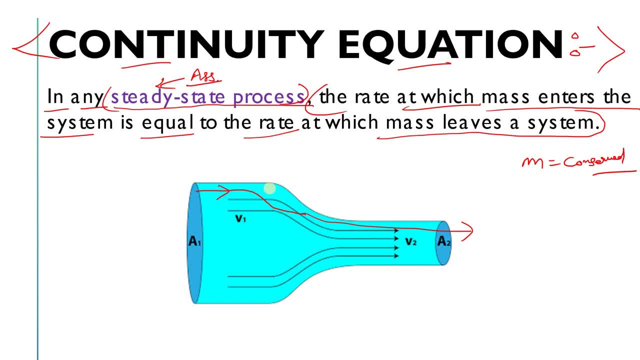 is your continuity equation. so before deriving the continuity equation: okay, so what is the like? this is the formula of the continuity equation, if you know that is, a1- v1 is equal to a2, v2. if your fluid is incompressible. mainly liquids are incompressible, so that's why we 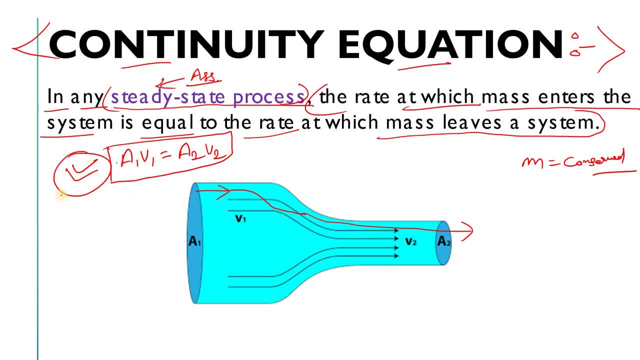 consider this equation. so how this equation comes into the picture, we will discuss about it. so before that, I would like to tell you some like terms which we are using here, let's suppose as a a1, v1, ok, so that terms. we must know that what. 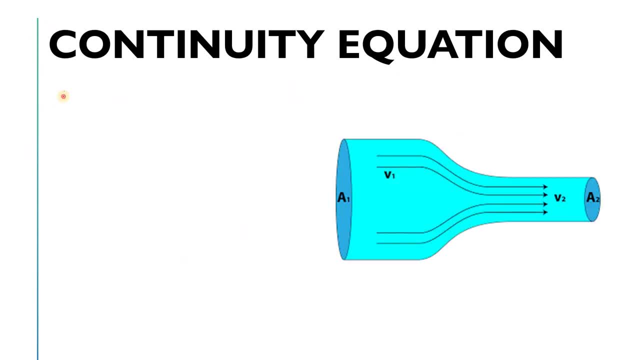 is this terms right? so I am just writing here what is a one here? actually the a1, the cross-sectional area. A1 is the cross-sectional area at 1.. Let's suppose this is your point 1 and this is your point 2.. Got it my point? So this is my A1.. So what will be A2?? A2. 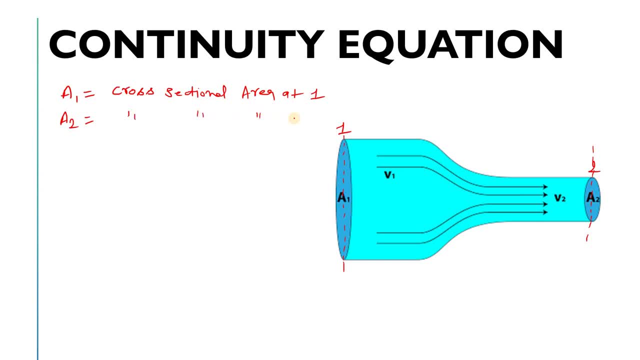 will be same cross-sectional area at 2. Right, Then. what will be V1?? V1 will be your average velocity at 1. Same. What will be V2?? The average velocity at 2, at 1, at 2. Right Now. 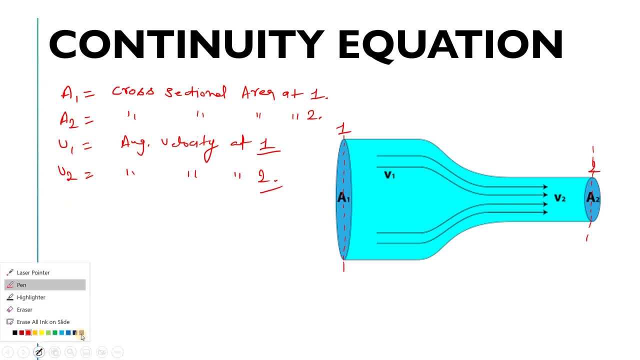 there is a one term as well which is very, very important And that you must know: that is your Q. Okay, So what is this Q? This Q is nothing but the volumetric flow rate, And it is also known as the weight of flow Rate. of Okay, This. 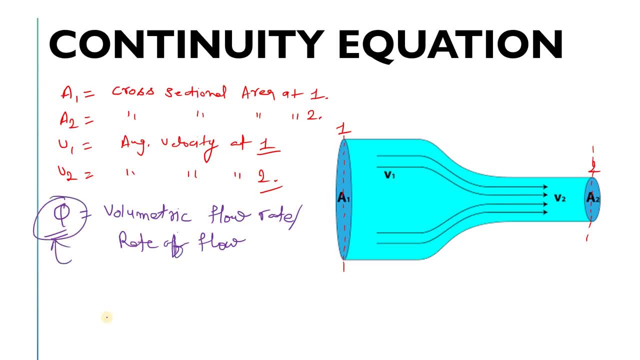 Q here with respect to fluid mechanics, Not heat transfer or thermodynamics. Okay, And in that case, this Q names is something else. That time this Q will be like your heat transfer rate, or this is simply heat added to the system or heat reject from the system. That is different thing. Right now, this is: 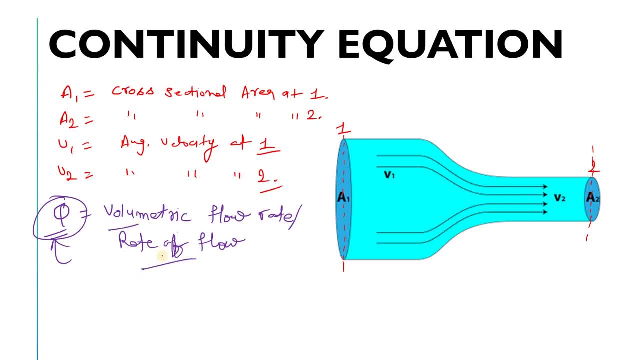 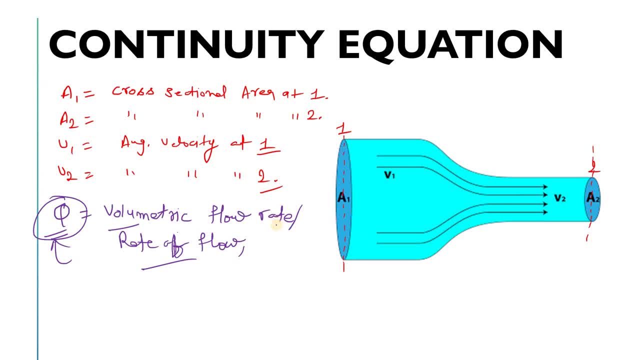 Through this cross sectional area. per unit time, Right, Because we are considering all we are saying weight. it means that per unit time, So it will be cubic meter per second. I hope you got the point, Okay. So what will be the unit of your area here? The area unit. 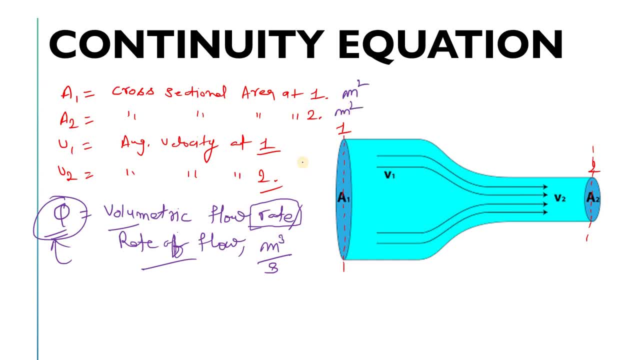 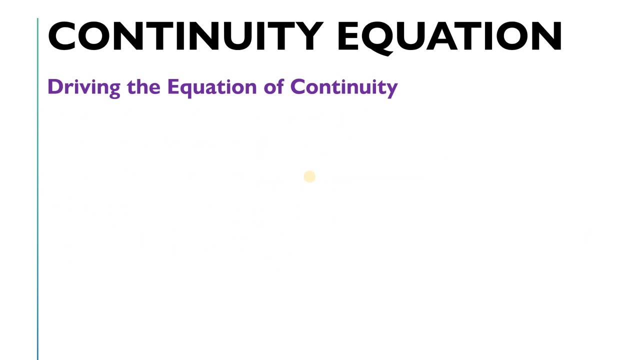 will be meter square Meter. why I am considering? because it is the SI unit. Okay, So velocity will be your meter per second and this will be also meter per second. So I hope that these terms are clear to you. Now we will proceed further, and now we will discuss about the driving. 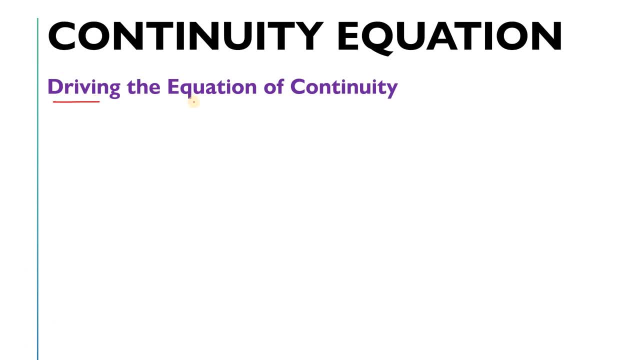 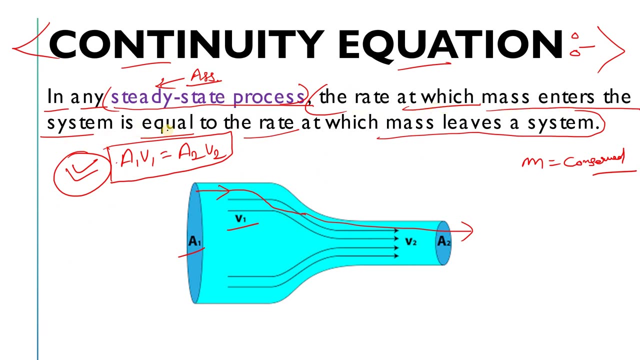 the continuity equation, So driving the equation of the continuity. So in our last slide we discuss about the statement of the continuity equation. that is, the rate at which mass enters the system is equal to the weight at which mass leaves the system. So means mass, the weight. 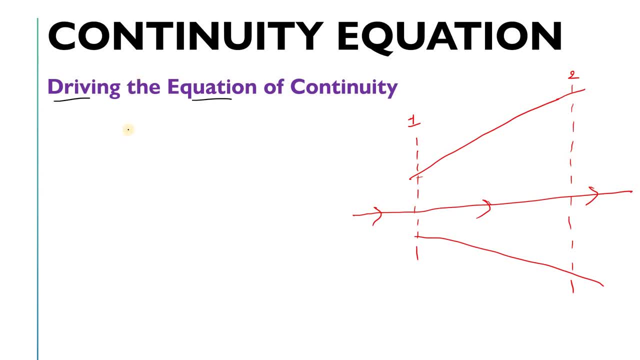 at which mass leaves the system is equal to the weight at which mass enters the system Means. we are here considering the mass flow rate, So m1 will be equal to the m2, that is the mass flow rate. Let's consider that at your A1, the area is A1. 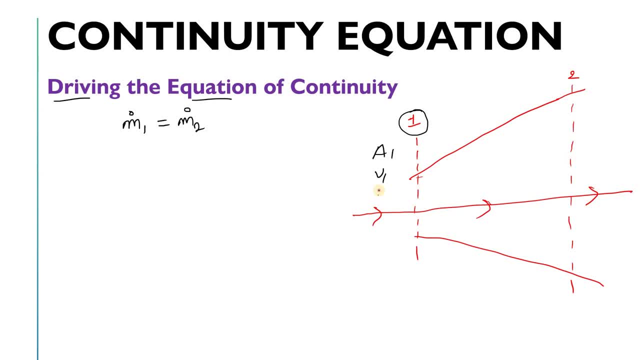 at A1,, the area is A1, velocity is v1, density is rho1 and the flow rate is q, Same A2,, v2, rho2 at your location, 2.. So how to calculate the mass flow rate and here the q. 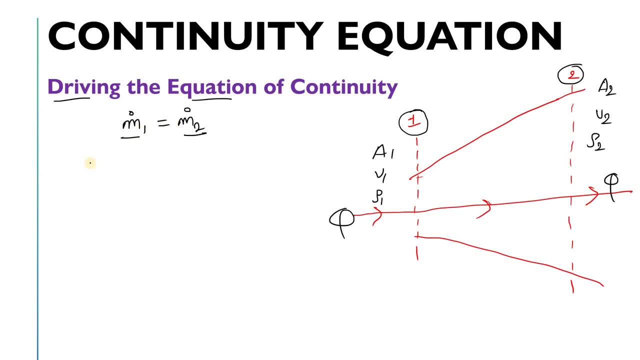 So how to calculate the mass flow rate. The mass flow rate formula will be: what is the mass flow rate formula will be: what is the mass flow rate formula will be vary in a又 m2. Ok, So in the last slide we called it velocity. 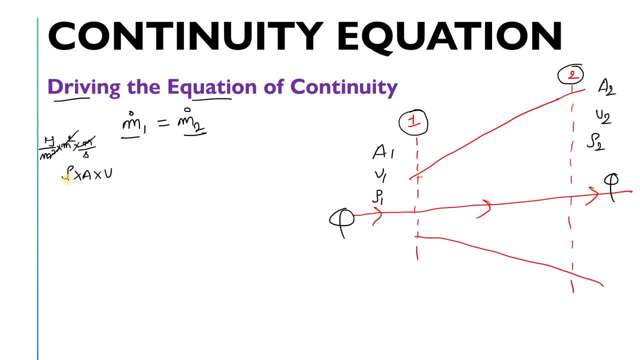 Rho, both of them equal to volume, and its at Cook's productrov. perfect2-lv is alright, So let's Baguio first and we can иo a high pressure of tension. 04, 05 and the So m1,. it will be your rho 1, a1, v1 will be equal to your rho 2, a2, v2.. 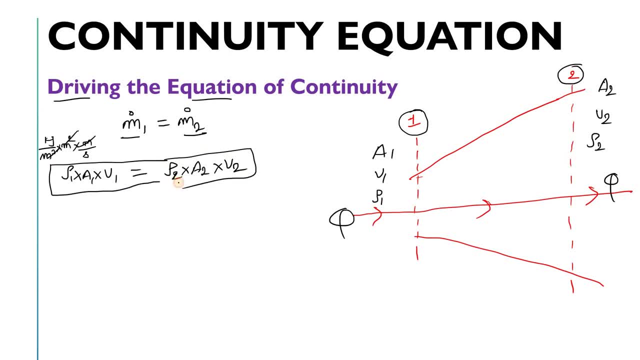 So this is your continuity equation, right? So this is your continuity equation. Now see if the water is flowing, or any liquid is flowing from this cross-sectional area, okay, from this pipe, you can say, from this tube or hose, you can say right. 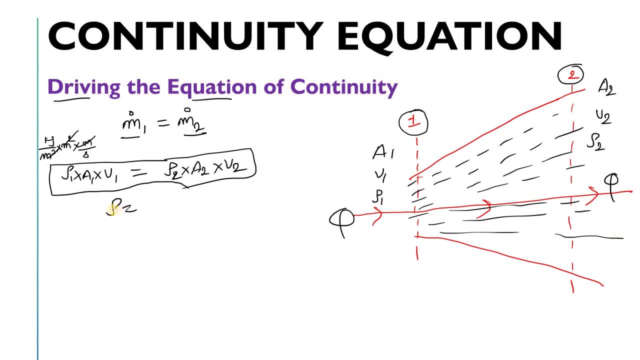 So now the density will be constant. At that time, your density is going to be constant, right? Can you let me in the comments box why density is constant in the case of liquid? So at that time the continuity equation will be known as: the a1, v1 is equal to a2, v2.. 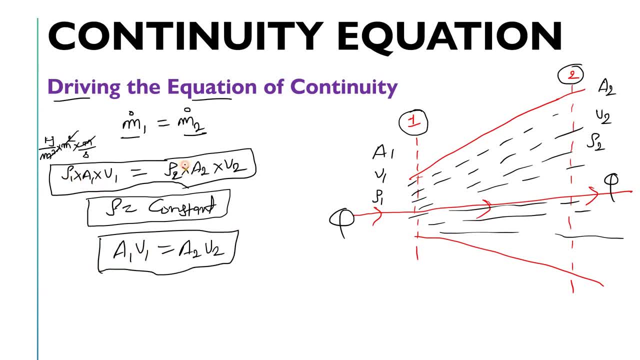 Got it my point? Okay, Because this portion is going to be constant, so it will be simply cancelled. Now, a1, v1 is equal to a2, v2, or simply you can say this is equal to q. That's why I have written here q. the q? q will be constant. 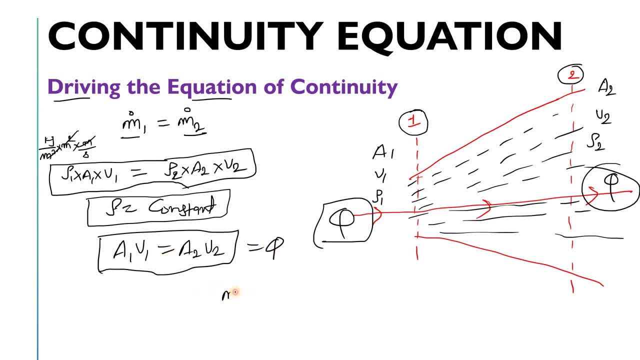 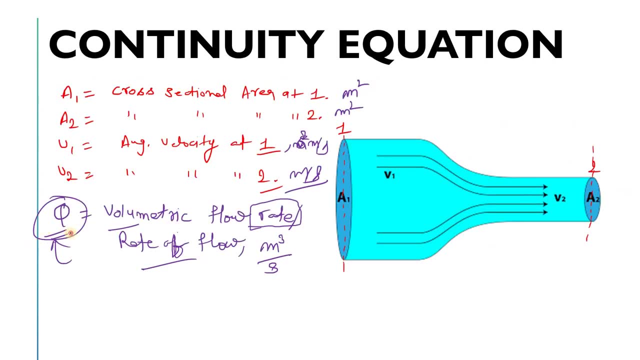 Got it my point Now. a1, v1 means your meter square into v1. is your meter per second, That is cubic meter per second, or that is your volumetric flow rate? We have, We have just discussed here, Okay. 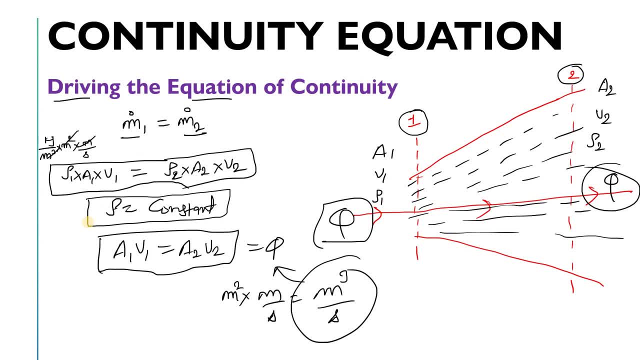 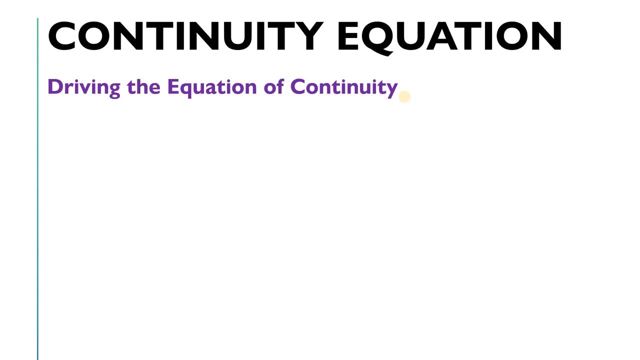 So I hope, the derivation of the continuity equation. you understood about it. Okay, This is very, very simple. Okay, Please do not confuse it. This is the just general form of the general derivation of the continuity equation, If you will like, if you will derive the continuity equation in the three dimension. 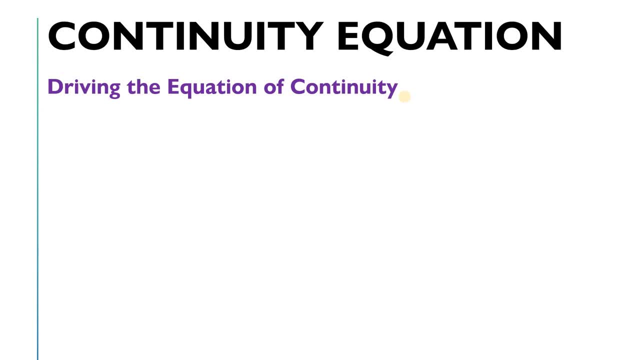 then you will get to know about some more useful information about it. Okay, So in this video we are not going to derive that. So the derivation of the continuity equation in the three dimension, if we discuss about it in the three dimension. 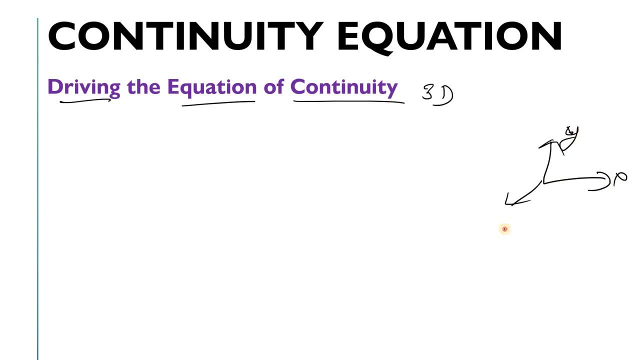 then you will get to know about the some more useful information. Okay, So there will be one derivation. Okay, If you will say so, I'll, in my next video, I'll describe that or I'll derive that continuity equation. Let me in the comments box. 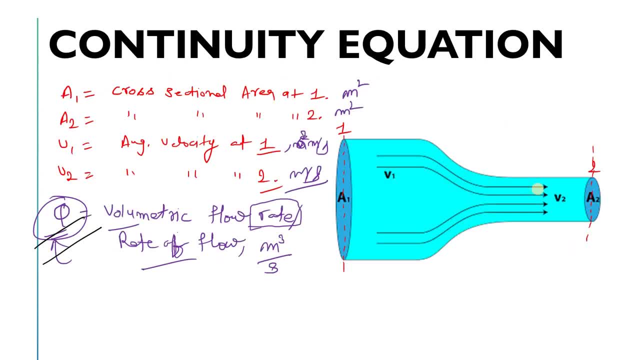 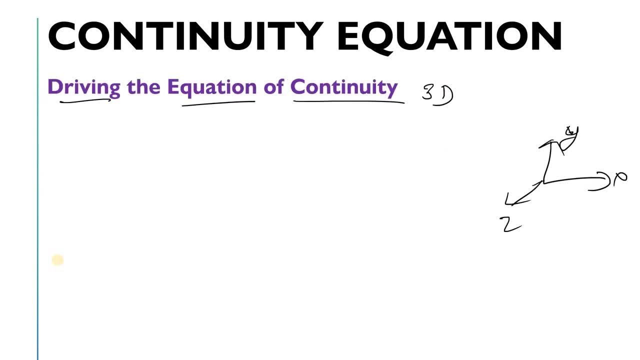 Okay, Or after that, the continuity equation which we have covered here, that is, also come from there. Okay, So that you must know, if you will, let me in the comments box, So I'll derive that equation and I'll also tell you that what is the journal equation? 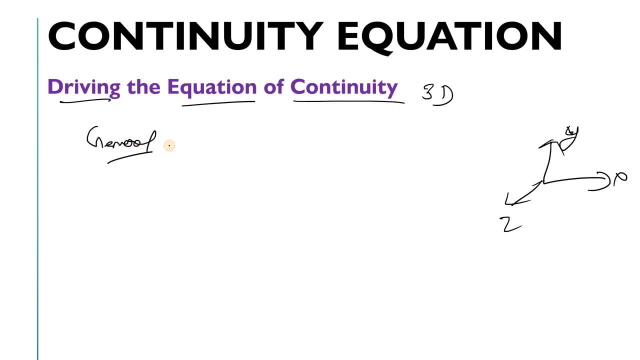 What is the journal equation You must know. And after that, what will happen that if the flow will be compressible, or what will happen that, or what will be the equation when the flow will be incompressible? What will happen that if it will be two dimension, three dimension? 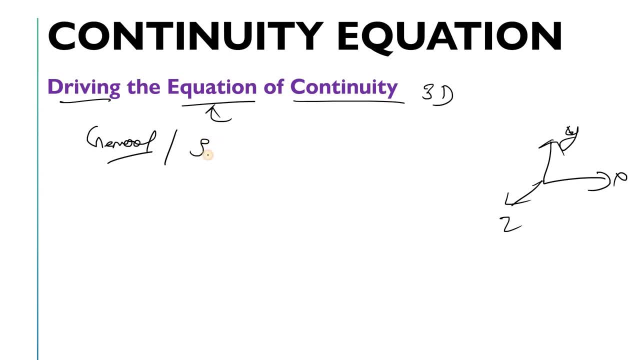 Okay, What will happen? that if the Fluid will be, you are at a steady state, Okay, So that all we can consider from there. That's why the continuity equation is also used in the compressible flow- uniform and non-uniform flow, viscous flow, unsteady flow- that we can use because that is a that is a journal equation. 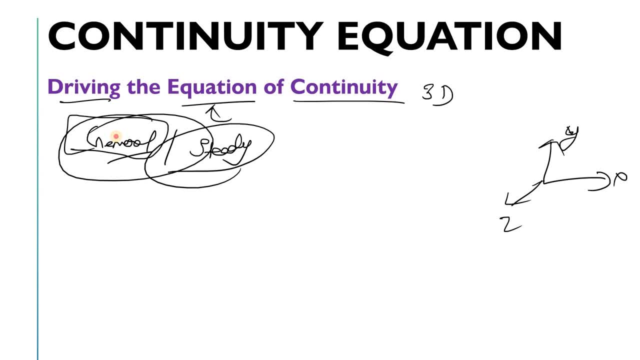 So let me in the comments box If you will tell me so I'll make the one separate video about it. Okay, So I hope that you understood the video. If you have any doubt in this video, please let me in the comments box. or, and if you are enjoying this video, if you are getting something new from this video, so simply subscribe core engineering YouTube channel so that I could make more videos, because it gives us the motivation, right. 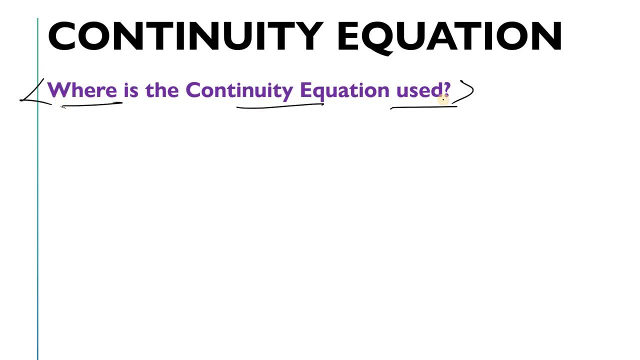 So now, where is the your continuity equation used? So mainly, as I already told, I have already told you that the continuity equation, Okay, The continuity equation gives us the useful information. Okay, It gives us the useful information about the transportation of the fluid. 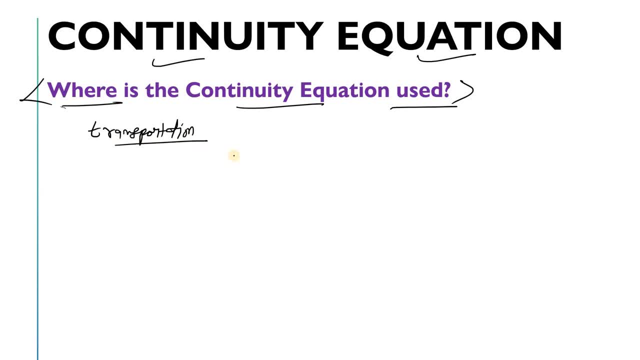 Okay, About the transportation of the fluid And simply you can say the flow of fluid and their behavior. Right, Let's suppose if one fluid is flowing through the, this pipeline, So it will give us the useful information about the its transportation. 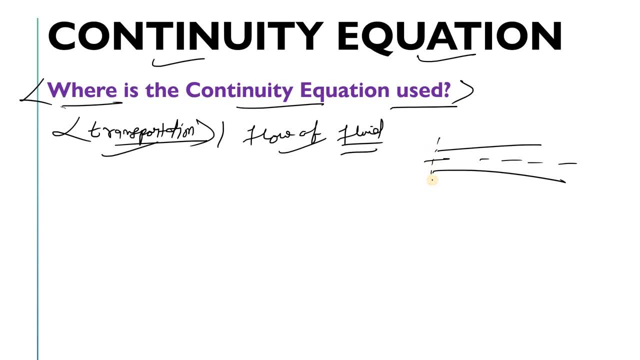 Or the flow of fluid. Okay, What will be the area here? what will be the area here? what could be the velocity here? right, Like this, right, And you can use this continuity equation at the pipe. you can use at the halls, you can use it. 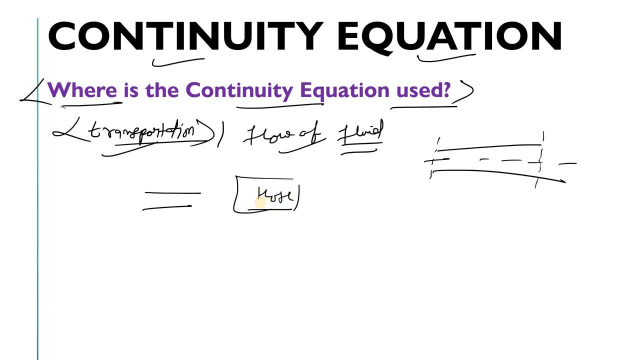 Okay. At the tubes, you can use it. mainly what I want to tell you that where this continuity equation use where your fluid will be flow Okay, Where your fluid will be flow Okay, And if you know the velocity And Q. 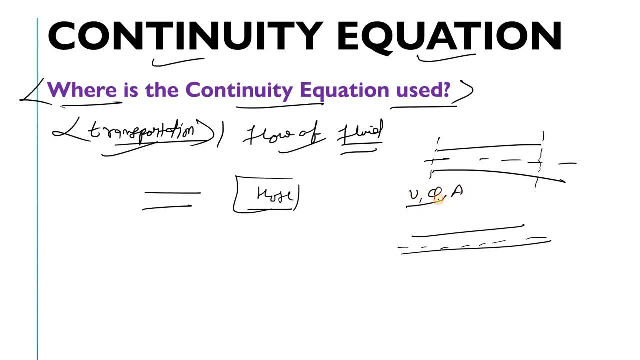 Okay, And area If any two values you know, so you can use any third value. So how useful is it? It is very, very useful while describing the flow of fluid and its behavior. Are you getting my point? So that's why it is very, very important. 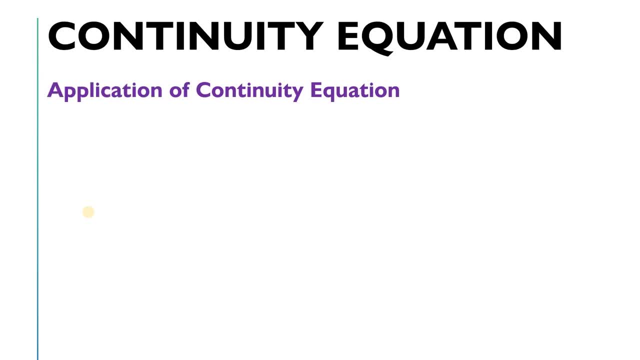 Okay. So now in the last, the application of the continuity equation. So simply, you can say, while calculating the velocity: Okay, We can use it. by line sizing, We use it Okay, Like that, Suppose, if you are dealing with. 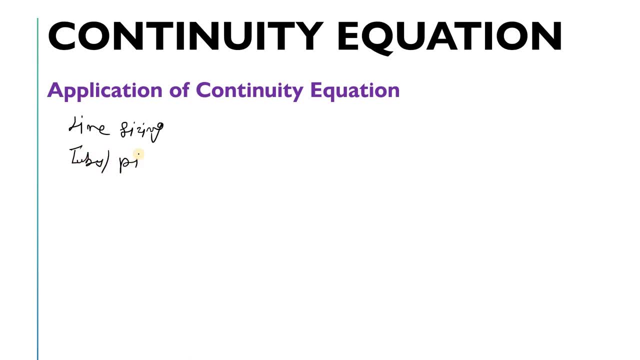 Tubes, Pipes, Halls- Okay. In civil, the river Okay. So there you can use the continuity equation Right To calculate or to know its behavior, to know the Behavior Of the following fluid. Got it My point? 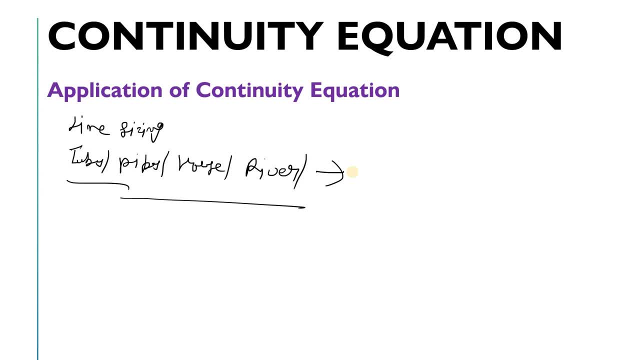 So that's why, also, the continuity equation is very, very used in line sizing. The continuity equation plays an very, very important role While calculating the size of the pipeline. Got it My points, And please let me in the comments box. 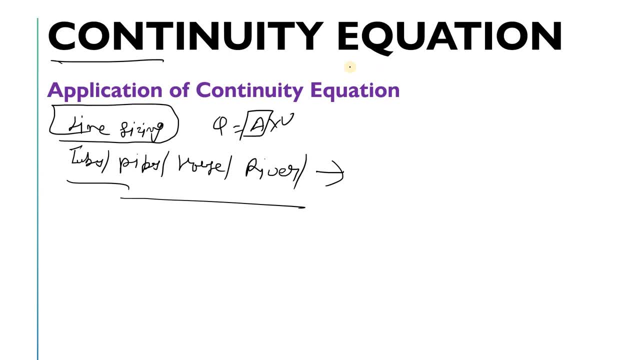 The most journal application of the continuity equation. The continuity equation is also tells us: from this equation You can simply say that the Q by A is equal to Velocity. So if you will increase the area, your velocity will be decreased. So you can simply see in your household. 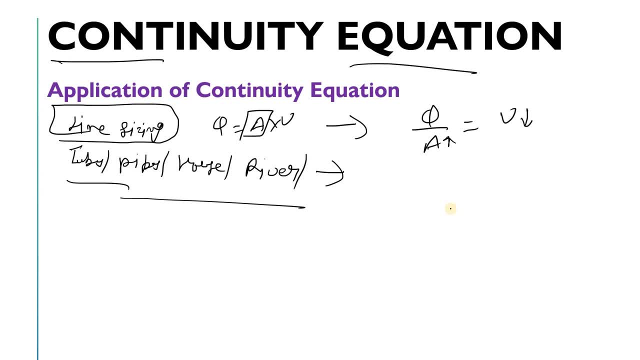 Okay, In your house application, in your daily life application, There is the pipe Which we connect with the tap Right. So this is your plastic pipe. And if I reduce the area, if I simply reduce the area, So velocity increases. 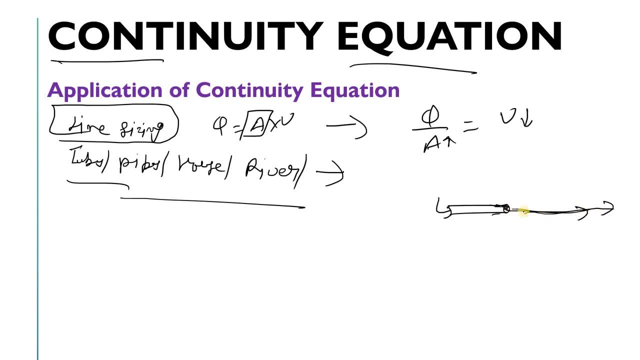 Your fluid will be go Like that: Okay Means it will go far away- Okay. So if you increase the area, So it is go like that: Okay, At the lesser Means it cover, the less Simply you can see the distance. 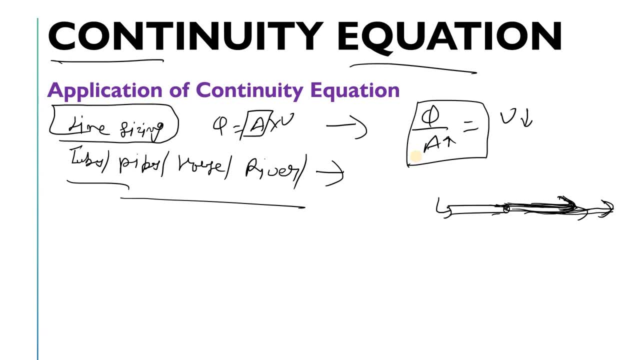 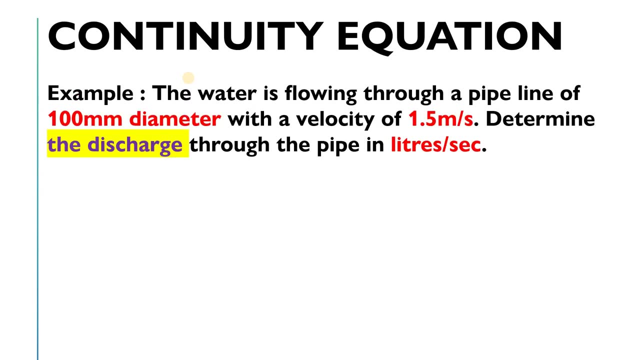 Got it My points. So this is very, very important while calculating in daily life example. Okay, So this is. its applications are wide in your daily life example As well as in the engineering application. Got it? So in the last, we will discuss here the example of the continuity equation. 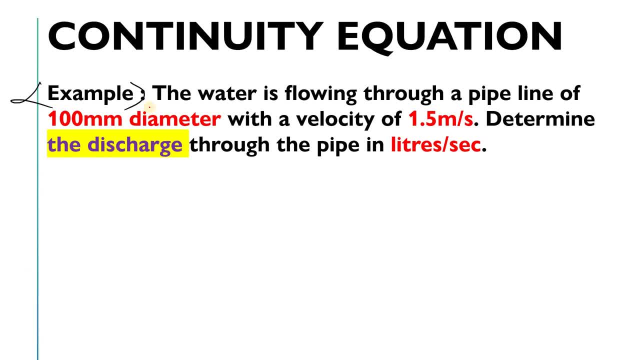 So let's see this example. Okay, So the example says that the water is following through a pipeline, Okay, Of 100 mm diameter, with velocity of 1.5 meter per second. Okay, Determine the discharge through the pipe in liters. 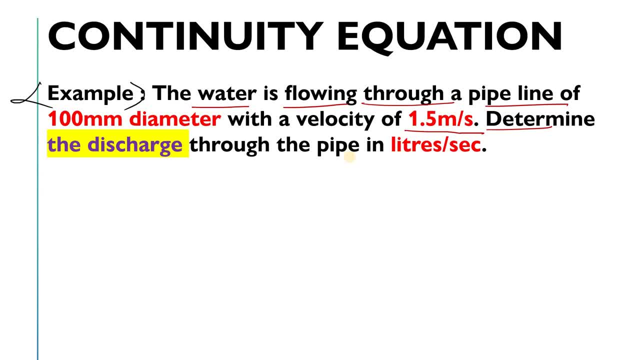 Per second. Okay, So I am not giving you the like exact answer here. Okay, I will not solve it completely, I'll just explain you the question. This is also very, very simple question. This is the dia, That is 100 mm. 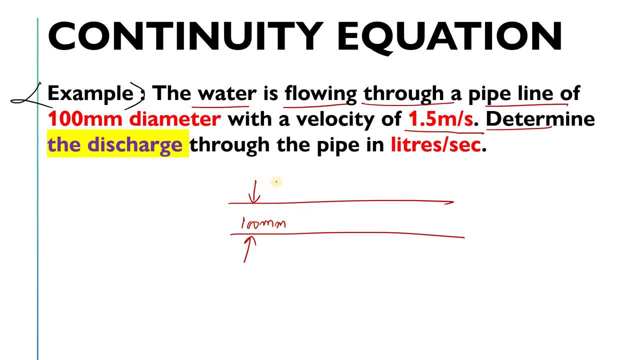 Right, The velocity, This is the dia, That is d, is equal to your 100 mm. So it simply you can calculate it at a Like in meter. So we know that 1 meter is equal to 1000 mm. 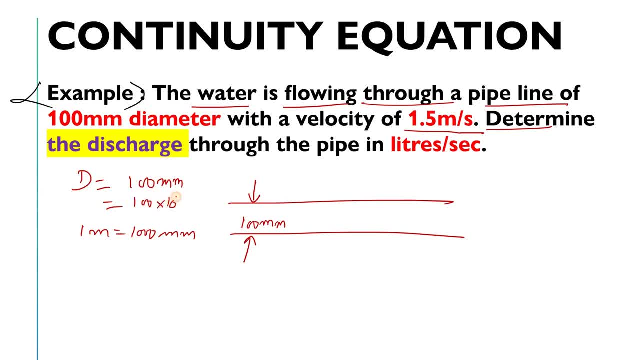 So what it will be? It will be your 100 into 10 power minus 3.. Now it will be in meter. Are you getting my point Right? So this is your dia. Okay, And with a velocity. 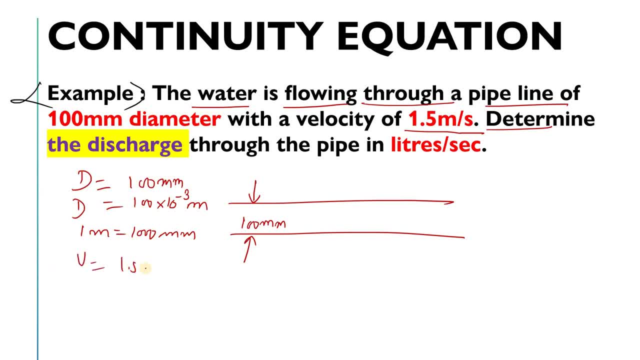 The velocity is your 1.5 meter per second. Now the unit is same, So right. So what you have to calculate? You have to calculate the determine the discharge through the pipe in liter per second. That is very, very important. 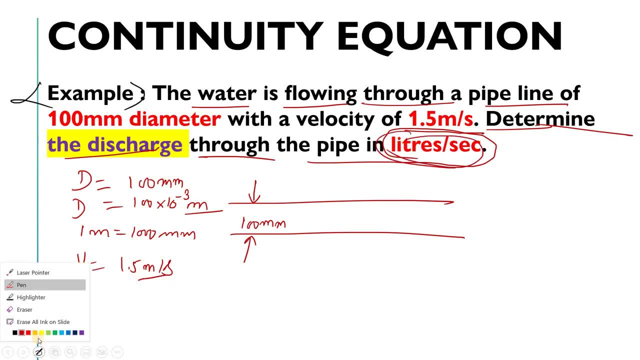 The unit conversion plays an very, very important role in engineering Right. So the q will be area into velocity. So what is the area here? The area is simply pi r square. You can say, or simply you can say, d square by 4..